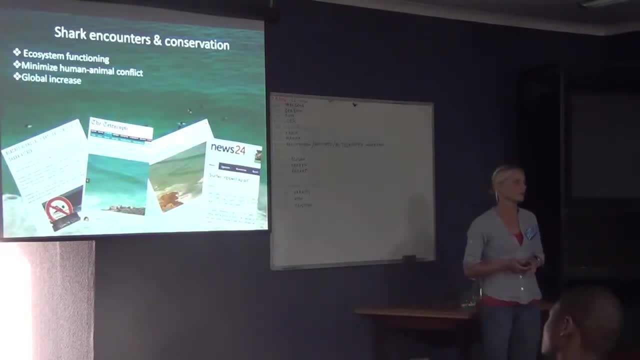 But as we've heard others speak before- that the shark encounters are a definite human-animal conflict. the shark attacks have been increasing globally and particularly in the Cape Peninsula itself. since the 1960s onwards we've seen an increase in shark attacks and also fatal shark attacks. 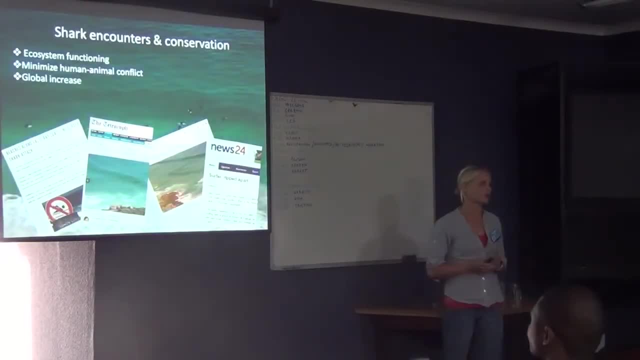 Also the shark attacks in themselves. it attracts a lot of attention and media and therefore have very negative effects on public perception and can negatively affect not only the economy of the areas in which these attacks occur, but also conservation of the species. So it's really important to understand more about these issues. 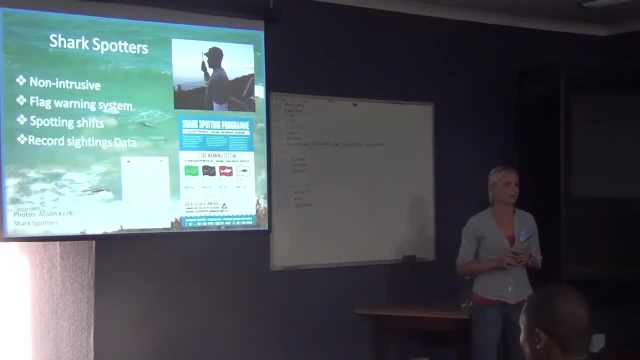 So there have been various mitigation methods in order to try and minimise these conflict areas, such as we've heard before: gill netting, perhaps drum lining, or even looking at some kind of electrical shark shield, Some of them less intrusive, others more intrusive a lot. 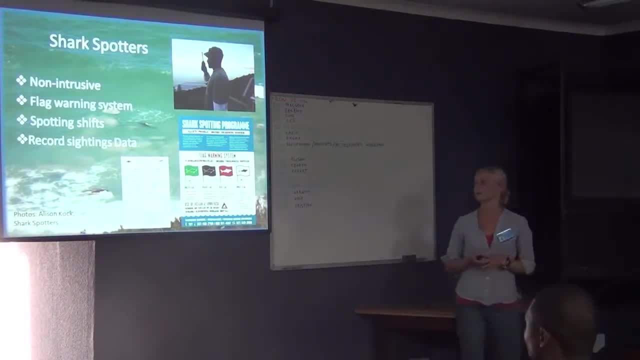 of them very detrimental to the environment as well as financially detrimental to the economy. So in about I think it was 2004,. shark spotters was implemented in False Bay as a non-intrusive method to try and mitigate this issue, And 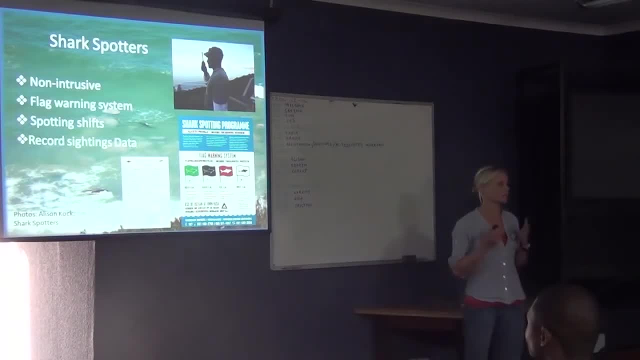 how it functions, or how it works is it's based on a flag warning system where two shark spotters are allocated to a spotting beach. One is situated on an elevated mountainside from a viewpoint, the other on the beach. Both are in contact with radios and have 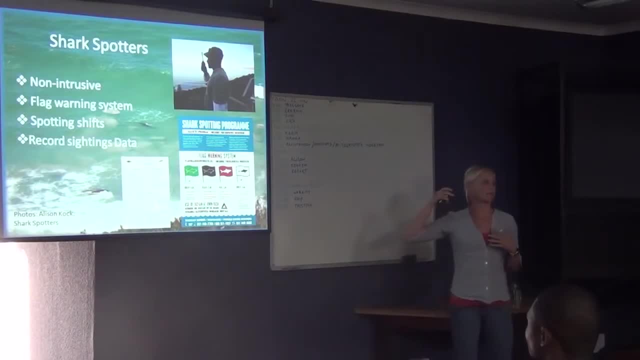 polarised sunglasses. and should the spotter on the elevated mountainside sight a shark in the area of the swimmers or the water users, he will alert the shark spotter on the beach. and he will alert the shark spotter on the beach. and he will alert the shark spotter on the. 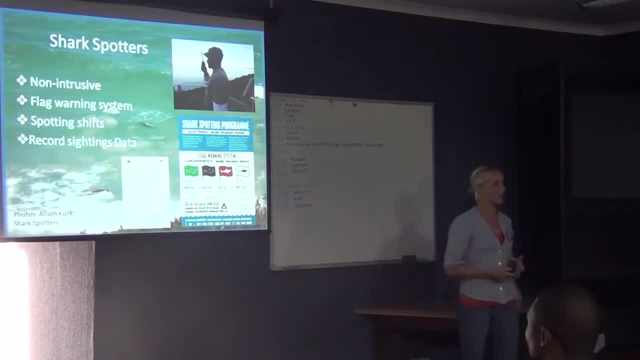 beach. he will then sound a siren and raise the appropriate flag to actually encourage the water users to exit the water. So to try and minimise that encountering, And in order to minimise spotting fatigue, shark spotters are divided into spotting shifts- morning. 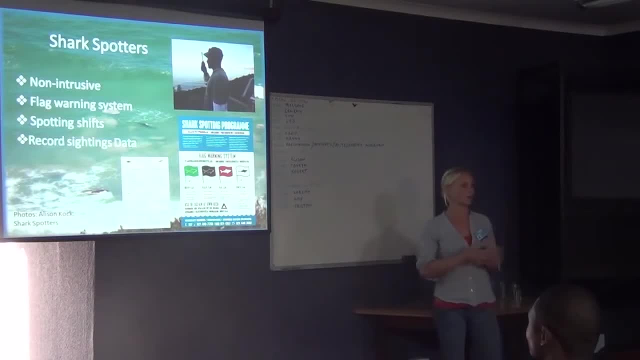 and afternoon shifts, and some are generally from about seven to one o'clock and one o'clock till seven o'clock in the evening. And not only do they try and warn water users of the presence of white sharks and get them to evacuate the water, they also collect very valuable. 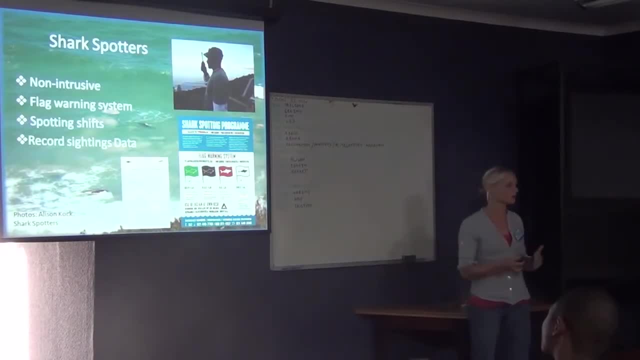 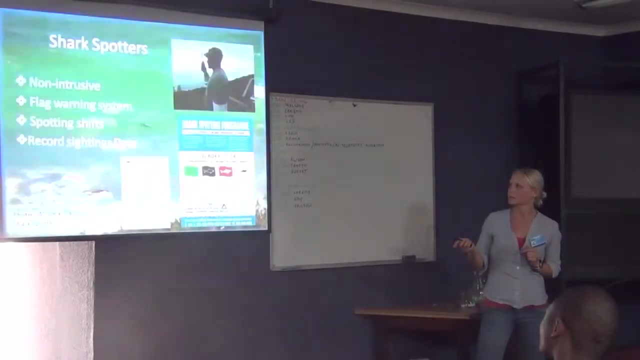 information on the shark sightings, so when it was sighted, how long it was sighted, the tracks of where it was going, so a lot of valuable data on these data sheets have been provided. The aim of this study was to use this data collected by the shark spotters to actually 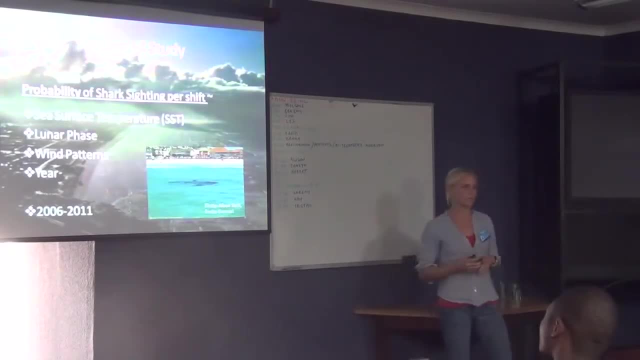 investigate a relationship between the probability of shark sightings per shift at beaches in False Bay in relation to environmental conditions and in relation to the location of the shark, factors such as sea surface temperature at the time, lunar phase, wind patterns such as wind speed and wind direction, as well as looking at a yearly trend of these. 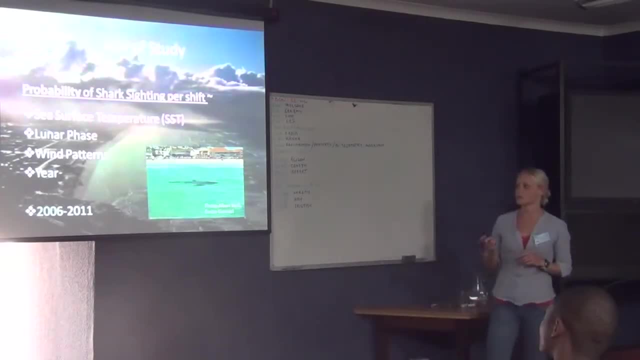 sightings along those beaches, And this study was conducted over the years 2006 to 2011.. And because it's difficult to distinguish whether a shark sighted by the shark spotters was the same shark or if it was different sharks coming and. 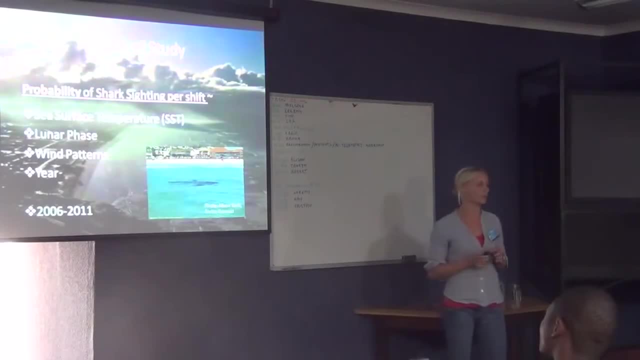 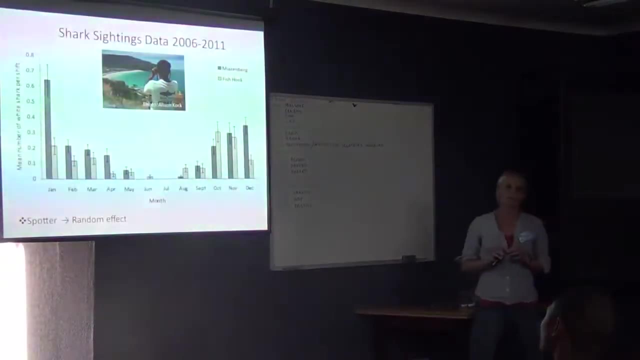 going. instead of looking at the amount of sharks, we actually took a binomial approach and used the actual probability of sharks. So just a bit of to touch on the shark sightings data itself. This study focus. there are seven. I think it's seven now right. 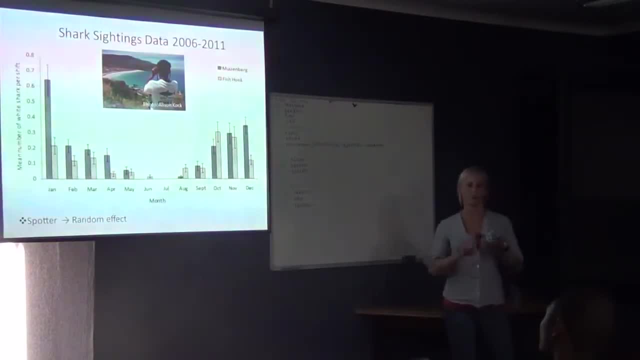 at some beaches which are in the shark spotters or have sharks. There's eight now. Is it eight now? Okay, so there are eight beaches now which have shark spotters allocated to them, But this study focus particularly on Musenberg and Fischer, because they have the most sightings. 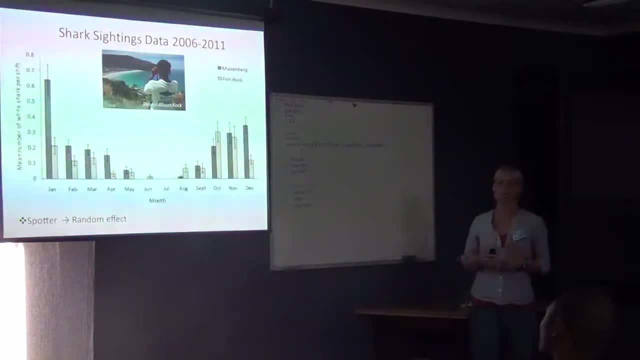 over the study years, so the best quality data and they also have the highest risk of encounters- that have had the highest risk of shark encounters over the years. So to give you an idea, this is the mean number of white sharks per shift across all the months of the year, for all the 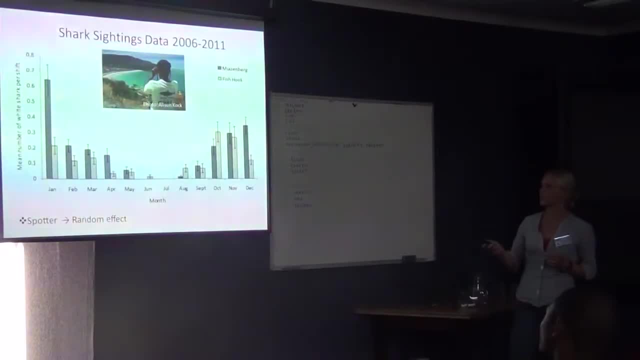 study years and, as you can see, there's a very clear seasonal trend, with increased shark sightings around the about autumn, spring and summer, particularly summer months, with very, very few sightings and poor sighting conditions in June, July and August and the winter months, and this has actually been confirmed by a 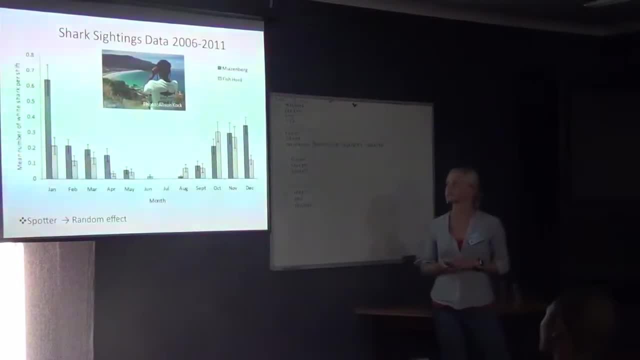 recently published study by Cockett Island 2013 earlier this year, which showed that, using acoustic tagging, that white sharks spend most of their time around Seal Island in winter months feeding on weaned pups and then tend to have a diet shift towards more elasmobranch and larger fish species, which 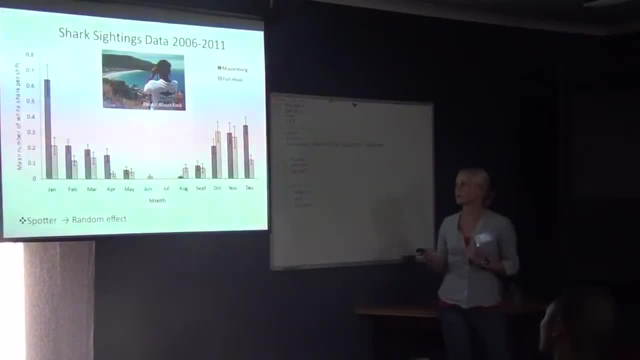 move into the area closer inshore in summer months. So therefore we excluded the winter months from the study to focus more on the summer months, when they actually are inshore for sighting, Because sightings data is very much dependent on the individual ability of the individual spotter. 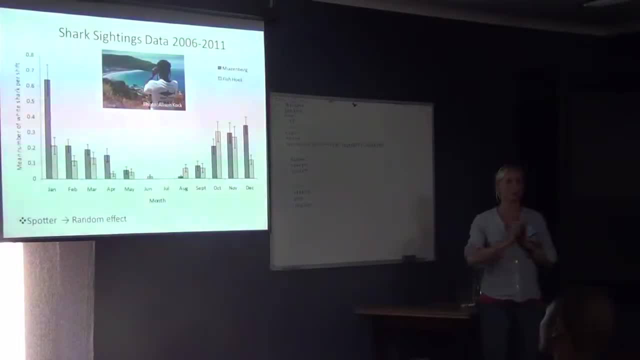 we have to be very careful about that. We have to be very careful about the individual spotter. So we chose to filter our data according to only include spotters which are done over a hundred spotting shifts at the designated beach, and we also included spotter as a random effect into our analysis to 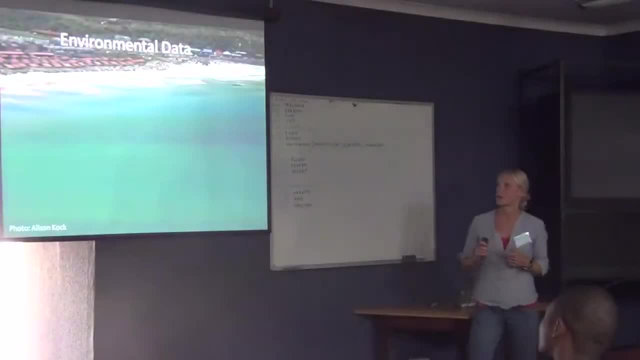 actually incorporate this. So our environmental data was externally sourced. We got the sea service temperatures from South African Weather Services and was provided in daily measurements from degrees Celsius by a handheld thermometer. Our lunar phase was provided by the South African hydrographics unit and we divided it into eight phases. so you have. 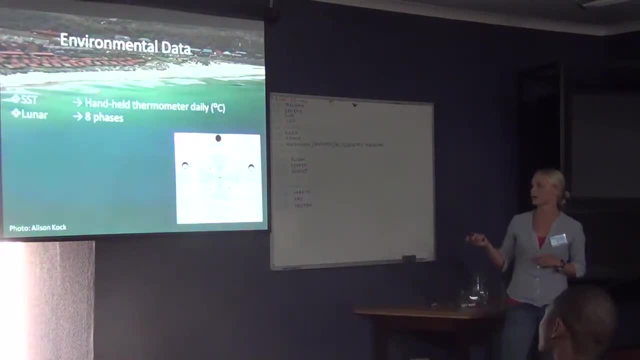 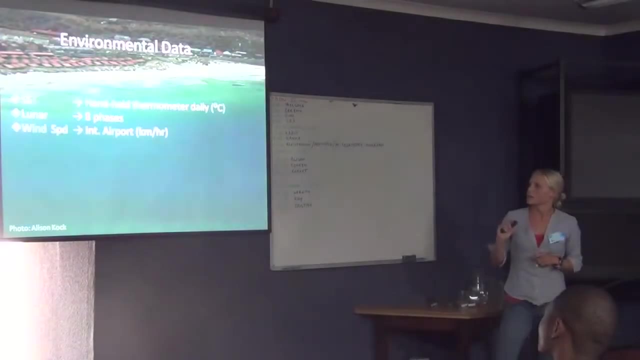 your common four phases- your full moon, third quarter, new moon and first quarter- and we divided this into further subsequent eight phases. within that, The wind speed was measured at the International Airport of Cape Town in kilometers per hour, which has been said to be the best representative for wind speeds in 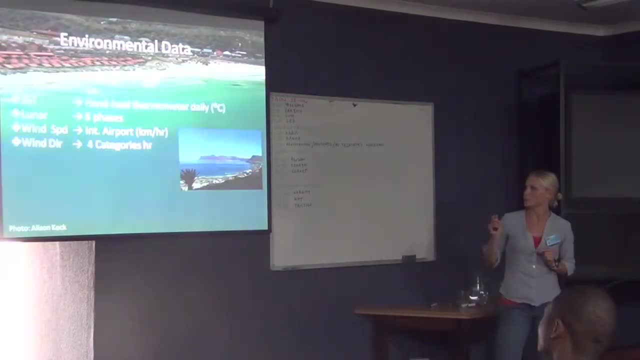 False Bay, and the wind direction was provided in degrees and was therefore categorized into four categories, namely onshore, offshore, cross-shore and longshore, for each beach individually, and both the wind data was provided by the South African weather service as well. So, in order to first touch on this data, we wanted to 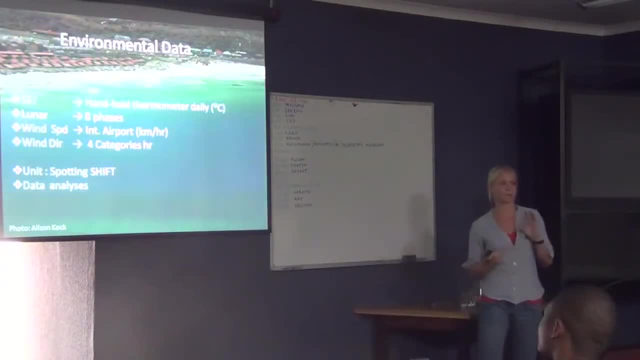 make sure that we had a consistent unit throughout our study and we chose spotting shifts of the morning and afternoon shifts I'd mentioned earlier we chose as our unit, So all of our environmental data was averaged for each shift and our shark site is allocated to these shifts. For the data analysis we wanted to see using 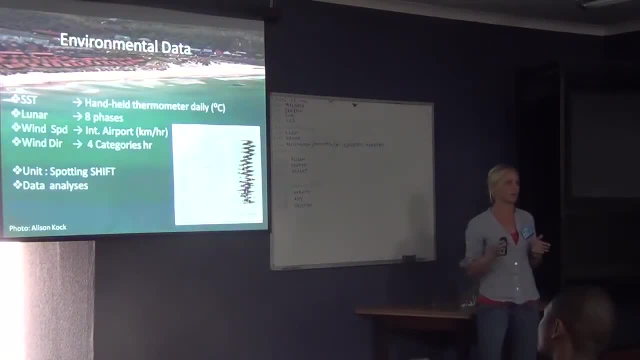 Cleveland dot plots and box plots whether the spread of the environmental variables over all the months of the year was a good spread, even when we took the winter months out, which it still showed, And we also used multi-panel scatter plots in order to identify. 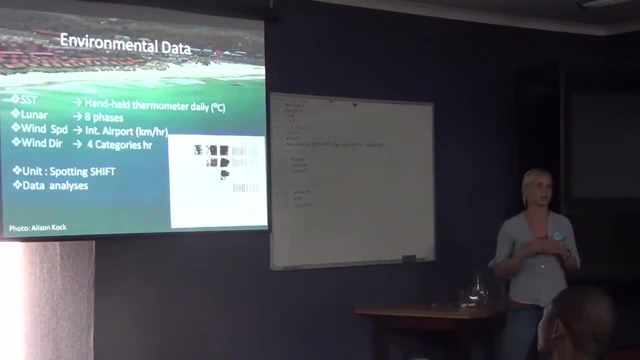 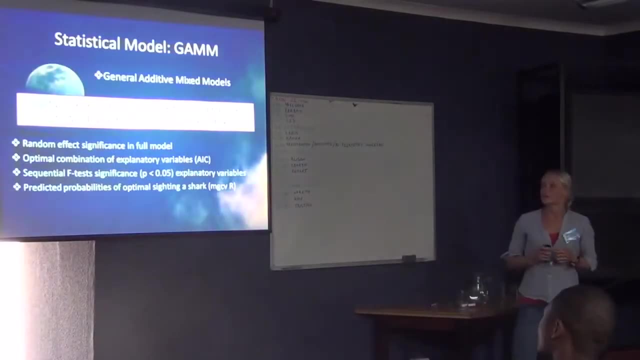 any co-linearity between these variables, which there was none, and there were no outliers. so therefore, all the mentioned variables here were included in the study. So in order to investigate the relationship between these environmental variables and our shark sightings, we used a statistical model known as a GAM, which is a general additive. 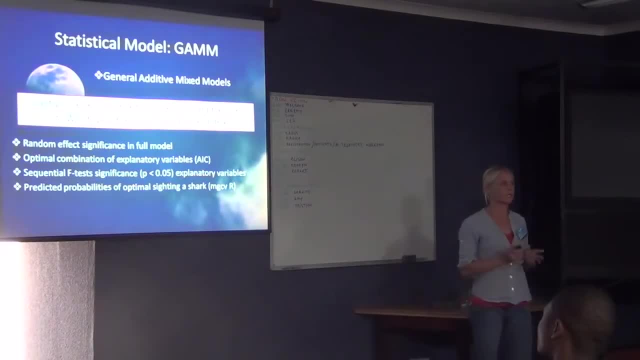 mix model And it is similar to our generalized linear models, but it is less restrictive to the underlying data And our data, particularly our shark sightings data, had a lot of zeros, So we had very non-normally distributed data, And generalized additive models are great. 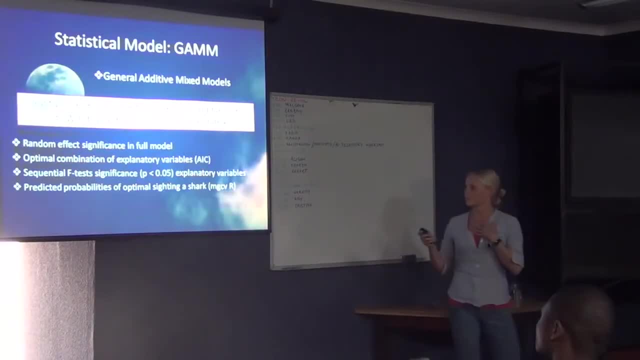 for non-parametric data, because they actually they replace the least squares with smoothing splines, which allows the model to better fit your data which is non-parametric. So this is the model which we our final model, for both our beaches And the logit function. 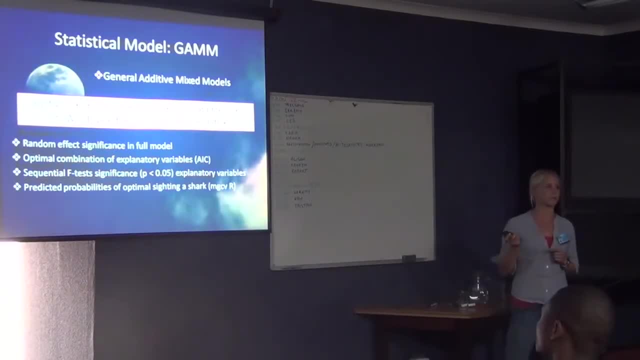 denotes the binomial link function, with p being the probability of sighting a shark at each beach. The year, sea surface temperature, lunar phase, wind speed and wind direction and shift were our explanatory variables. We added in shift as looking at time of day. 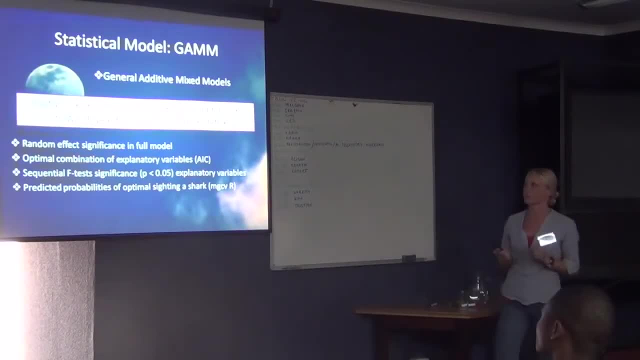 so, whether morning or afternoon shifts, if there was a difference affecting the probability of shark sightings And alpha being our random effect of the spotters which had been included. All our f's shown here are our thin plate regression splines, which we use as our smoothing. 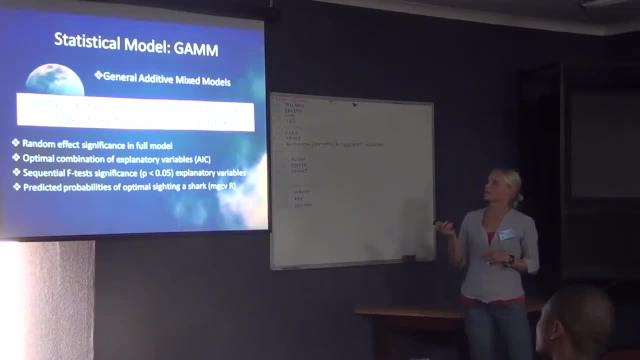 functions in this model. So, in order to get our full model for both beaches, we first included our random effect of the spotter into both models to see whether it was significant, which it was, so therefore we left it in both models- And to find the optimal combination of each one of these explanatory variables to our 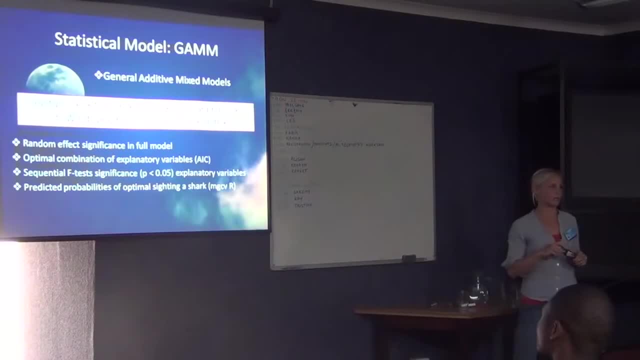 link function. we used the k-th information criteria with the lowest k-th information value, indicating the best combination of explanatory variables. Therefore, thereafter we used a sequential F test to actually test the significance of each one of these two. So we would then. 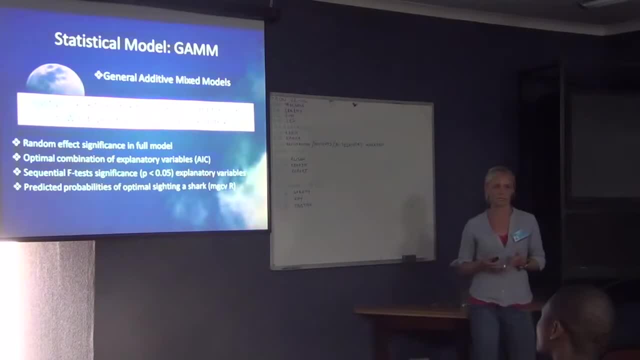 these explanatory variables and how that might affect the probability of sighting a shark. And we actually took it a step further in actually using this model to predict the best optimal times and probabilities of sighting sharks at both beaches. And all of this was done in the MGCV package in R. 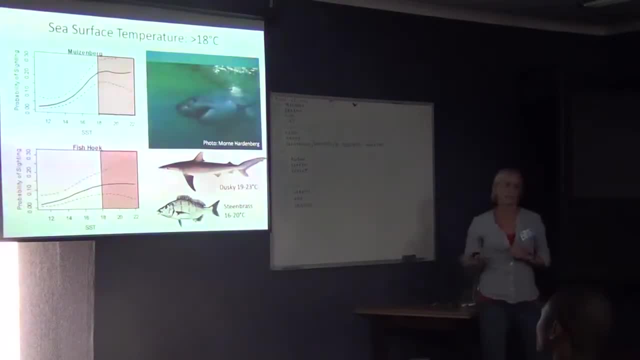 So our results: The sea surface temperature was highly significant for both Musenberg and Fischerhoek, showing very similar trends, with increased probability of sightings towards 18 degrees Celsius, with a peak around 18 to 20, and then after it then stabilizes. 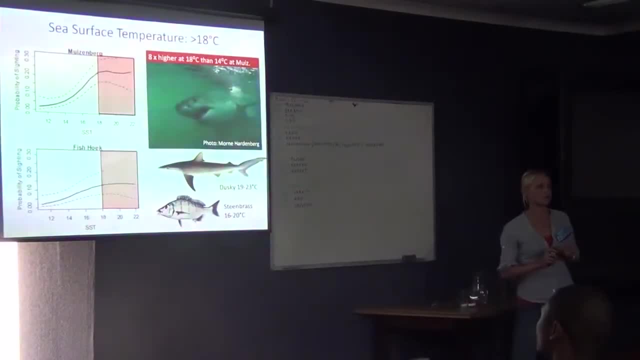 And our model predicted an up to eight times higher chance of sighting a white shark at 18 degrees in comparison to, for example, 14 degrees at Musenberg. Our reasons for finding this trend. we first, there were two options in our mind. 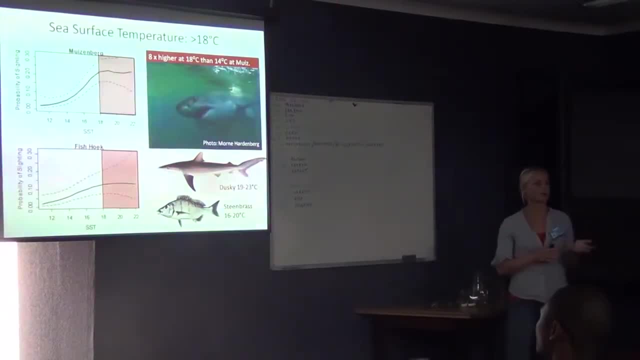 It was either. you know, it's the physiology of the white sharks themselves, so their own preferences for these things. It's either it's these temperatures or it's their prey, And white sharks have a very wide tolerance range in terms of temperatures, from about 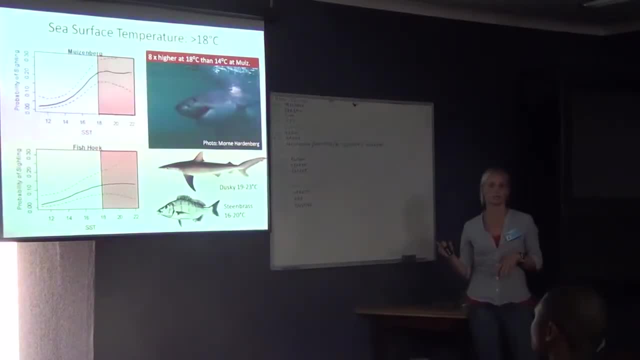 0.5 degrees Celsius in Alaska all the way up to 22 degrees Celsius in California. So it's very unlikely that they're going to be limited to such a narrow range by their own tolerances. They're also able to increase their internal body temperatures by up to 15 degrees. in comparison, 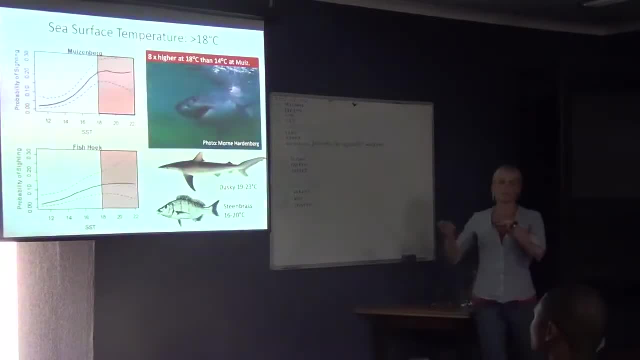 to the external temperatures. So again, very unlikely. So we turned to their prey to see if we could find any answers there, And we found that they were very, very tolerant. They were very, very tolerant. We found that white sharks in summer, as shown, have a dietary shift towards more lasmobranch. 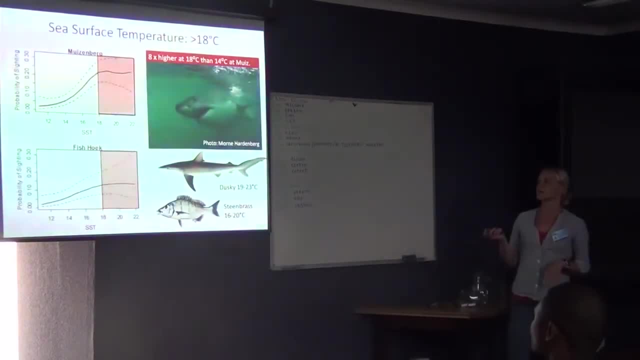 and fish species which move into false bay in these times. Dusky sharks, for example, are known to migrate down from Pasoola Natal to escape the warm waters up there, And white zebras also spend a lot of time in summer inshore. 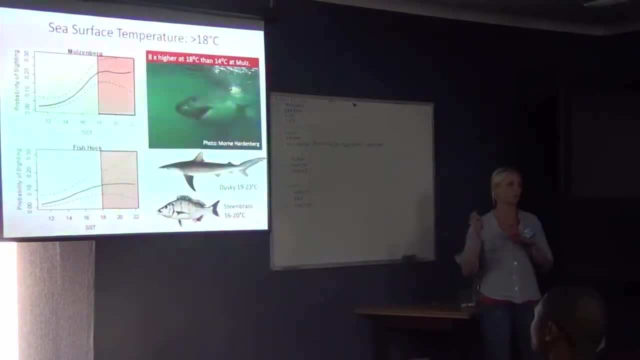 And these are very common prey species. These are just a couple that I've mentioned, But we've actually found a whole list of prey species from white sharks which show very similar temperature ranges, in this time in false bay. So we're quite certain that it's the you know the you know the you know the you. 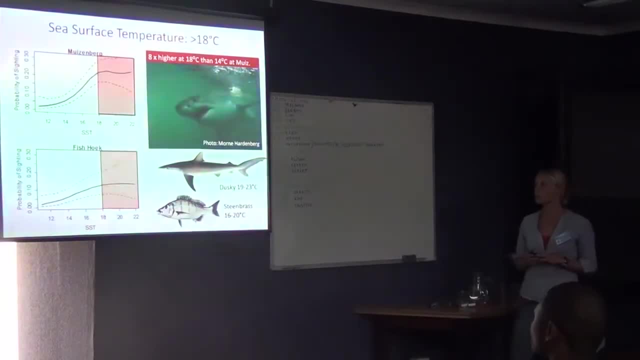 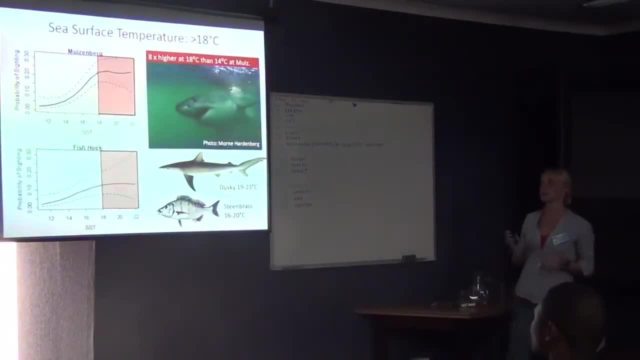 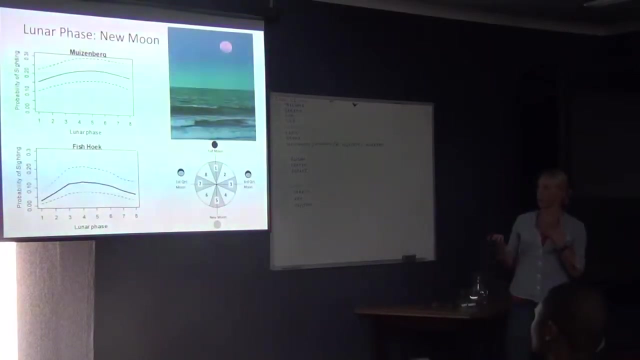 the So we're, so we're quite about to expand. this New Moon was the highest probability of sighting white sharks- 4, 5, 6 being here down here. 4, 5 and 6 around New Moon. 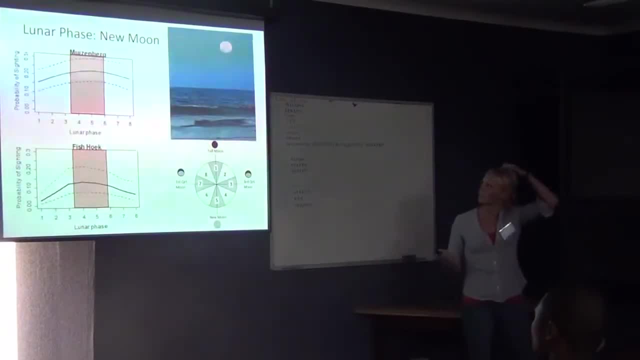 the lowest probability at full Moon And our model predicted up to 4 times higher chance of sighting a shark during New Moon at Fish Hook in comparison to full Moon. Now, Moon phase is known to provide very predictable patterns in the marine environment which have a great effect on all behavioural functions of marine organisms. 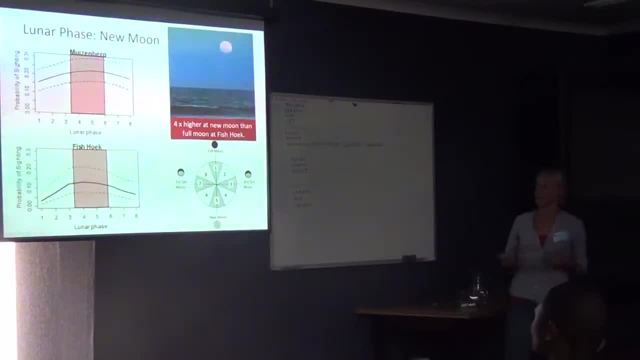 Such as reproduction or migration or aggregation, And it has actually been shown in various other studies: One in False Bay looking at seal colonies, which showed an increase in success of predation rates around New Moon In California, where they said that it was the camouflaging of the white sharks. during low light intensities which allowed them to better have hunting success on their northern elephant seal prey Or even in Australia they had shown that great white sharks caught catches in nets. closer inshore of juveniles was again higher at New Moon in comparison to other Moon phases. 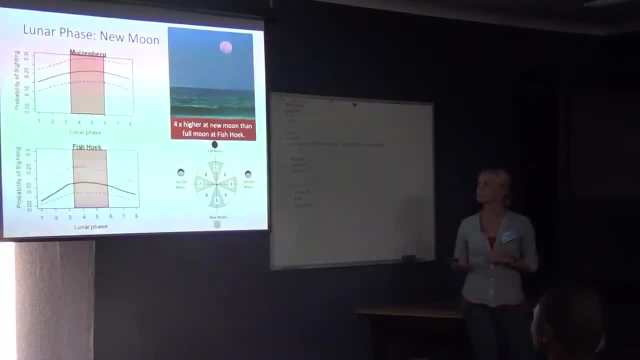 So there are other studies out there to support our findings. So we do. I mean, although the mechanisms in False Bay itself are not known as to why are we finding this trend? we think it's most likely due to hunting strategies or increased hunting advantages. 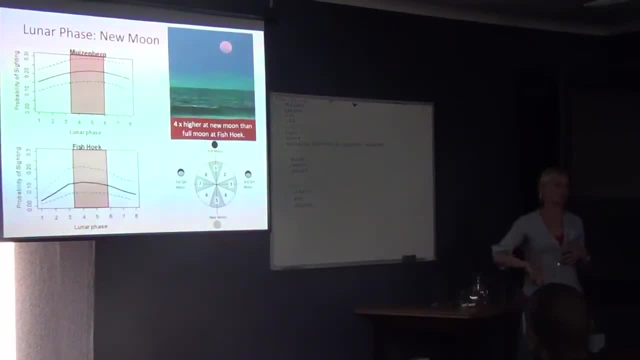 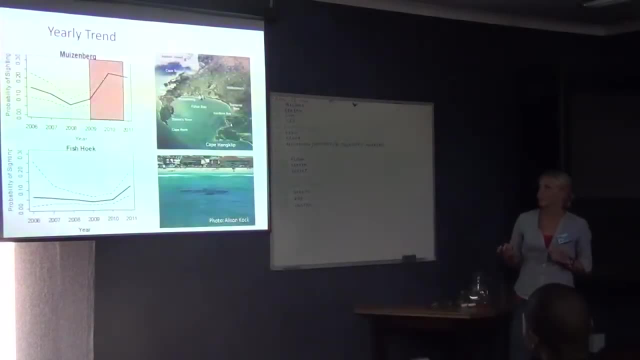 and movement of increased food availability into that area during New Moon. Our third most significant variable was the trend in year And we found that there was, for both Muesenberg and Fischlger around 2009-2010, an increase in shark sightings. 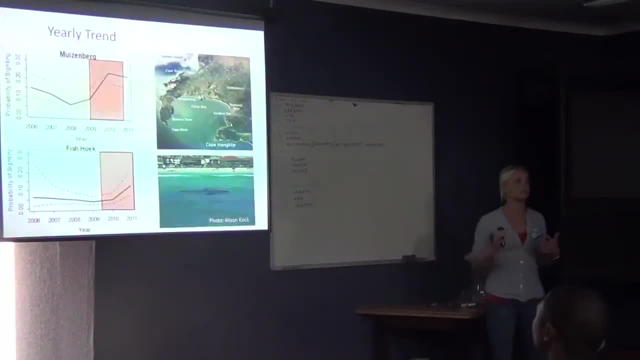 We did investigate whether there was a change in temperature over these years and we found that there was no significant difference in water temperature between any of our years. So the water temperature stayed relatively the same. But reasons for actually finding this recent increase may either be due to: 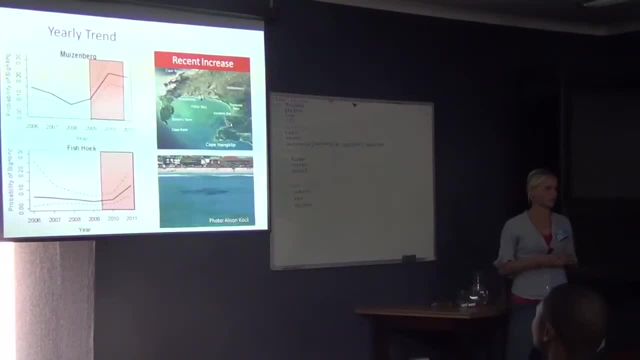 an increase in the actual population numbers of white sharks in False Bay And, as Alison mentioned earlier, Adrian is actually doing a population estimate at the moment, so it would be quite interesting to see those results. Or it could also be because they've been protected by law for the last couple of years. 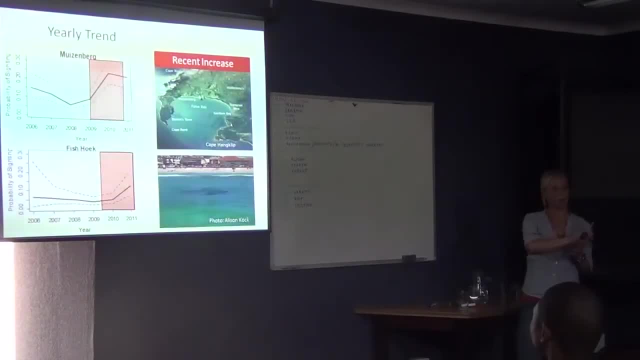 so it would seem to make sense. Or it could be one individual shark which is just using that area more frequently, or it could be other sharks moving into the area or into False Bay over time. So, although it's not really known why, we're seeing this increase. 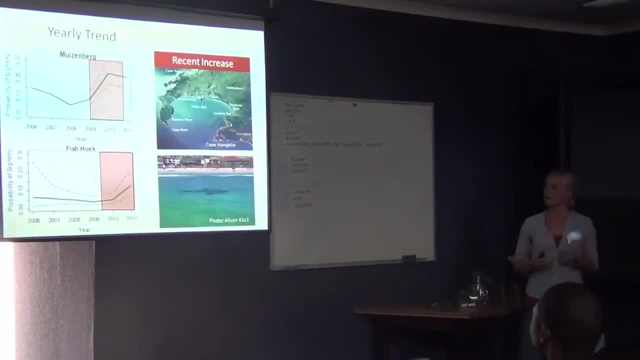 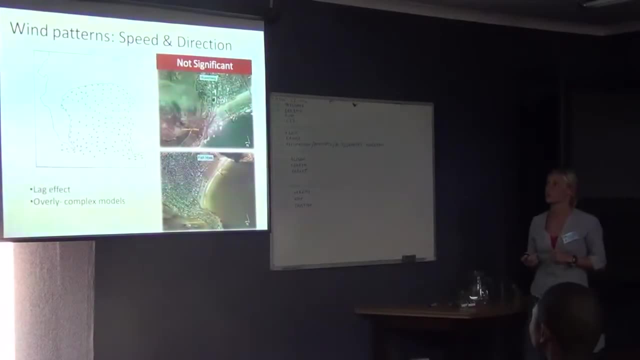 it just highlights. it's really another need for more research into this area. Our wind patterns, wind speed and direction were not significant for either Muesenberg or Fischl in our model And although this seems strange, we understand that it's most likely due to a lag effect. which we did not include in our model. So what happens in False Bay is we have the south-easterly wind which blow really strong throughout the summer, and a couple of days in a row, and then they track warm water along the river. 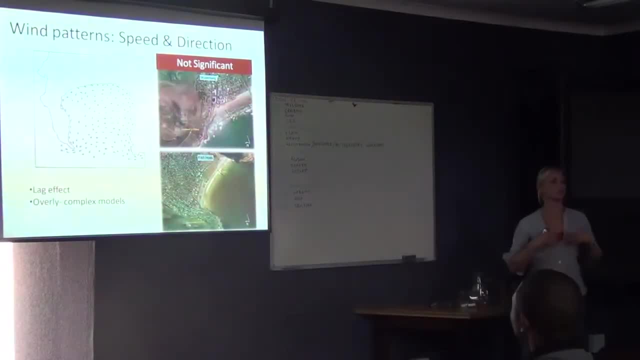 And then the coastline, which leads to algal blooms and increased fish movement into the area. But this is usually a lag effect, so it usually takes a couple of days for this to actually come into effect, And we didn't include the lag effect into our model because it over complexes the model. 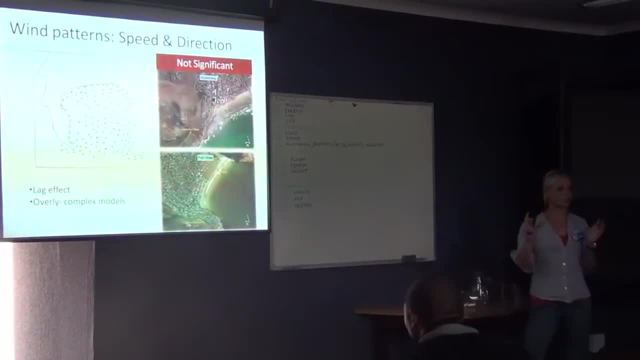 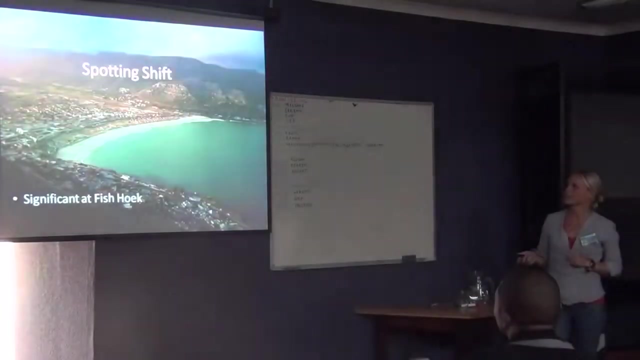 The GAM actually really struggles to separate the effects of each individual term when it becomes too overly complex by including interaction terms and all sorts of lag effects, So this might be something which could be looked at as a whole, separate project. Spotting, shift or time of day: we found only significant for Fischl. 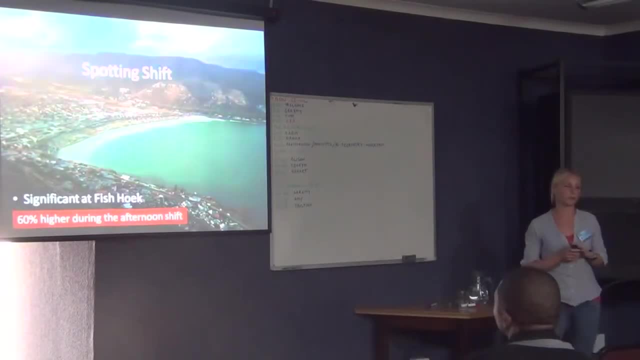 which was 60% higher chance or probability of sighting sharks at Fischl during the afternoon shift, which I found was quite interesting. now, having heard Jeremy's talk, But perhaps because we're not quite sure about the actual behavioral mechanisms that Fischl gets- 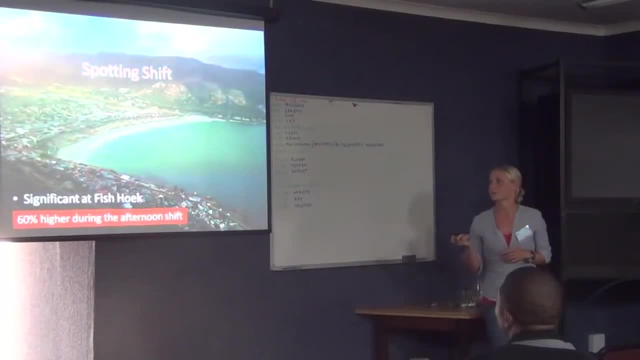 and more data needs to come in on their movement here. it might also be due to geographic positioning of the beach itself. So Musenberg and Fischl are situated differently geographically, And the viewing angle from Fischl's spotting point is northerly. 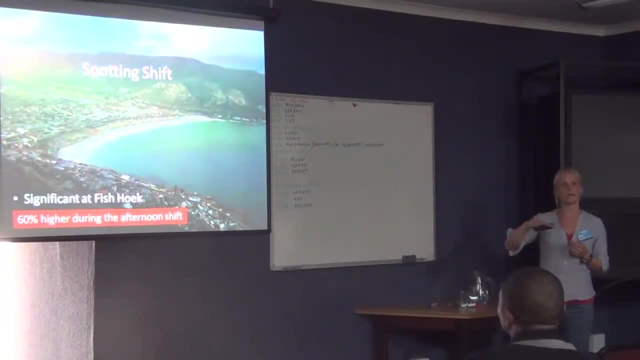 which is where the sun rises, So it might struggle with glare in the morning and that kind of stuff. But I think what would be quite nice would be actually, because this is a very purely quantitative study- it would actually be nice to almost do a qualitative study as well with the shark spotters. 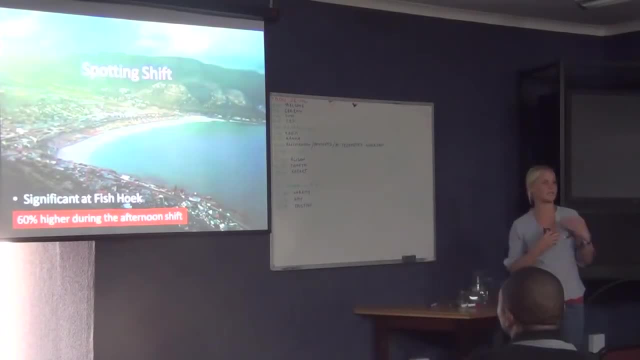 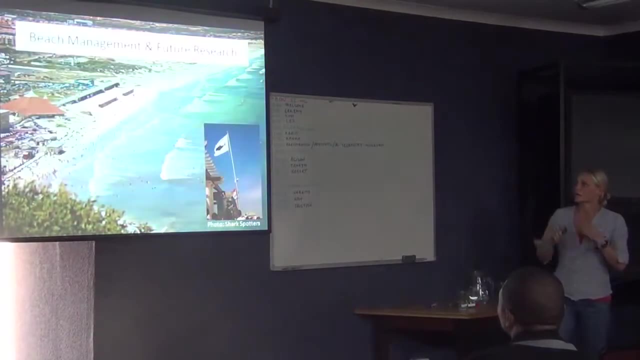 to almost understand, you know what are they seeing in those moments or how are they struggling to capture data in those times. So this might be another thing that could be expanded. So how is a study like this put into management and applied? Shark spotters have communicated the outcomes from sea surface temperature. 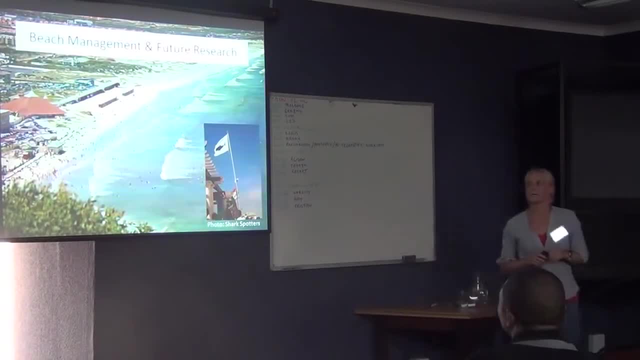 and lunar phase to the public through various media. It's too early to tell whether bather awareness has been changed through such an outcome, but bather numbers are being recorded by shark spotters and continuous monitoring and implementation of this model in the future, as well as bather numbers.